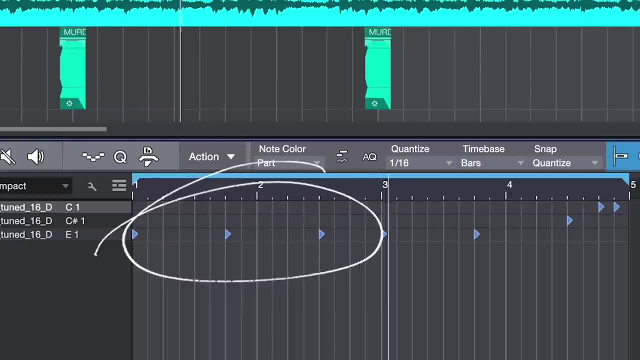 And this is what I like to call slow Tresillo. The ratio of 3, 3, 2 is still maintained, but it's up to you to decide if you want to use it or not. This is what I like to call slow Tresillo. The ratio of 3, 3, 2 is still maintained, but it's up to you to decide if you want to use it or not. 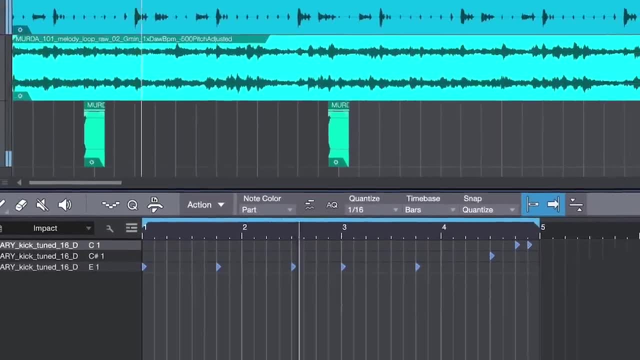 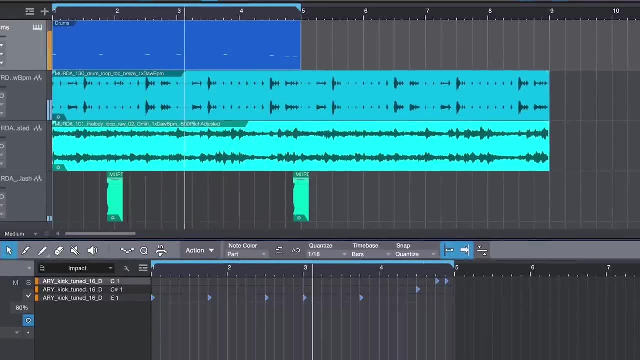 This is what I like to call slow Tresillo. The ratio of 3, 3, 2 is still maintained, but it's up to you to decide if you want to use it or not. This is what I like to call slow Tresillo. The ratio of 3, 3, 2 is still maintained, but it's up to you to decide if you want to use it or not. 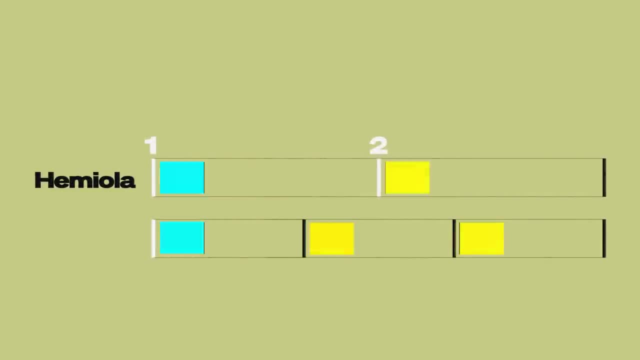 The next rhythm that changed my life is known as a hemiola. This is the most basic polyrhythm, which, if you're unfamiliar, polyrhythms are when two or more rhythmic feelings are stacked upon each other. The hemiola is a three against two feeling, meaning one rhythm is playing three. 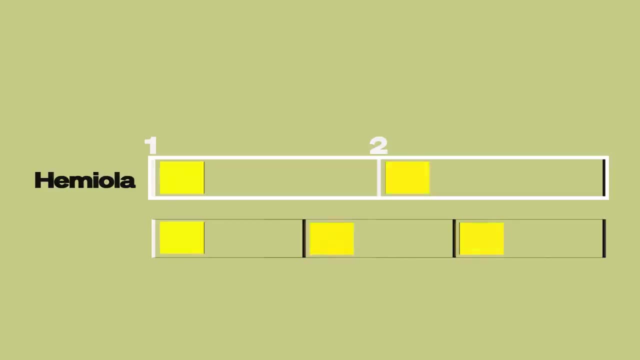 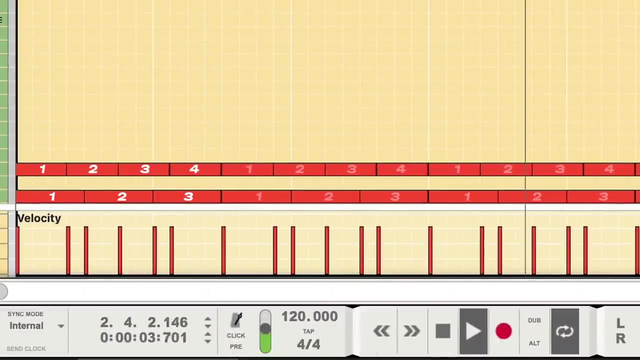 even beats in the same amount of time as the other rhythm plays two beats. Hemiolas really opened up the world of polyrhythms for me. Another popular polyrhythm aside from hemiola is 4 over 3.. Here's an example of a hemiola in a melody: 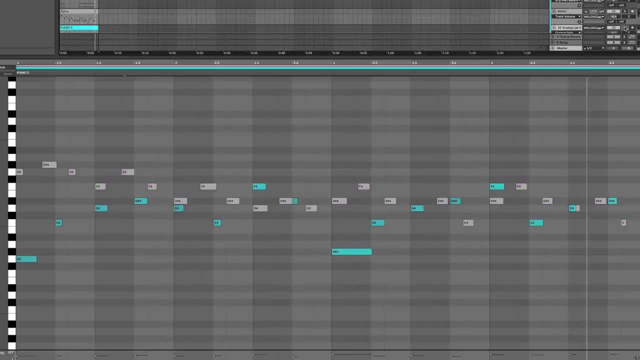 Maybe you're looking for something that sounds like a siren. what is it? Maybe you're looking for something that gives you a good tune that's not just a Riley. Oh, I didn't know you could play a r writing tune If you merge the two layers of the hemiola into one rhythm. 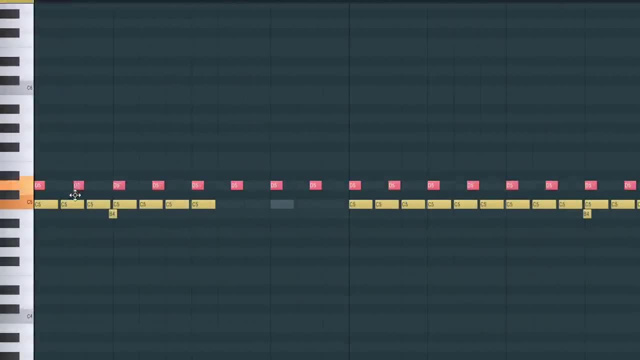 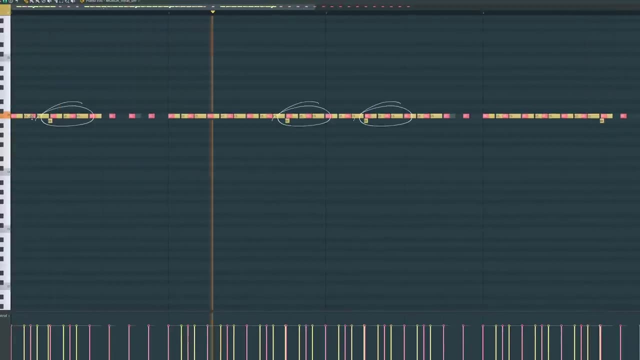 it creates the foundation of the rhythm of my favorite rudiment, the flam drag. In addition to this, there's the band and the arpeggio, And if you're a music lover, it's also a good thing to have a band and a arpeggio. 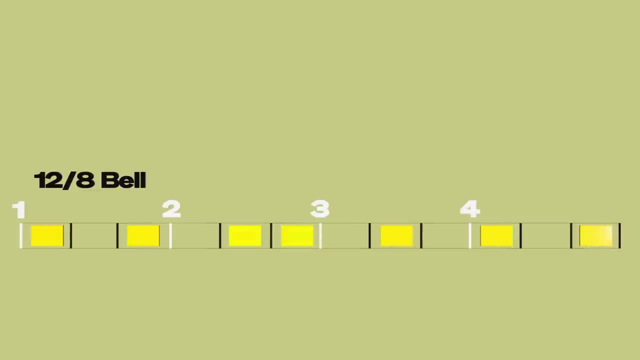 Out of the two. the band is a key to the beat and it's important that you have a atmosphere of sound. You get to play with both over 3 and 6. And if you merge the two layers of the hemiola into one rhythm, it creates the foundation of the rhythm of my favorite rudiment, the flam drag. 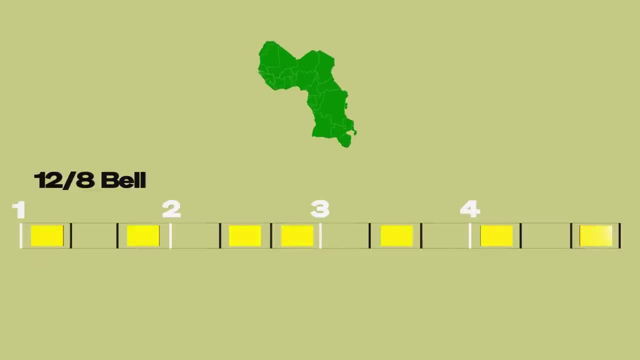 bell, also simply known as the bell pattern, in Central and Western African music. This pattern really opened up my eyes about rhythmic perception. It's almost like an audio illusion, as in it can be perceived in two different ways. You can hear the rhythm in four, or you can hear the rhythm in 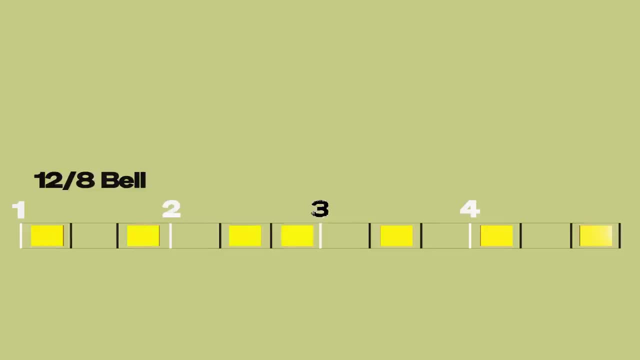 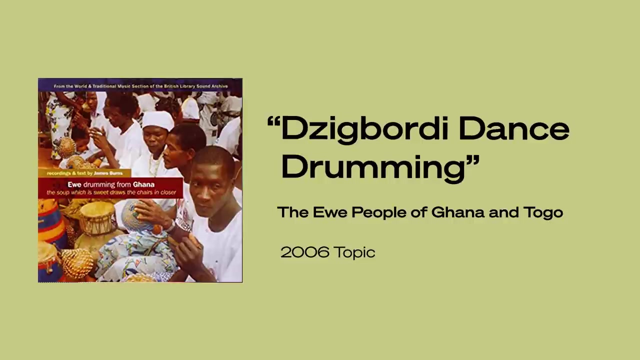 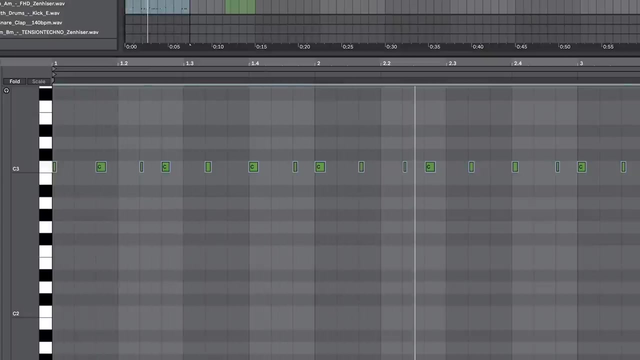 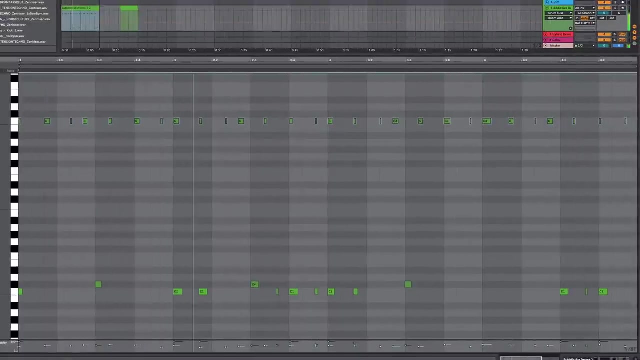 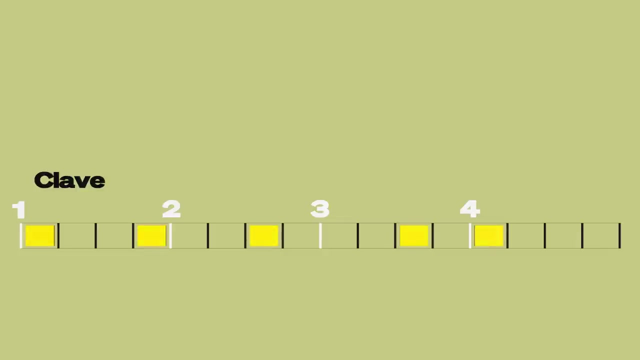 three. Let me show you. Here's an example of bell pattern in traditional A-way drumming. I personally like using this rhythm on my hi-hats or my ride. cymbal Clave, which translates to key in Spanish, is a fundamental rhythm in many Afro-Cuban genres. 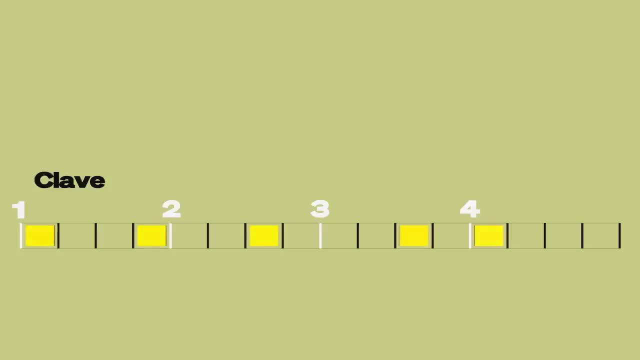 as well as Sub-Saharan African genres. The first two beats you should already recognize, since it's our first rhythm, Tresilla. However, Clave is a four-beat rhythm and there are actually four variations. The default one and most common is Son Clave. 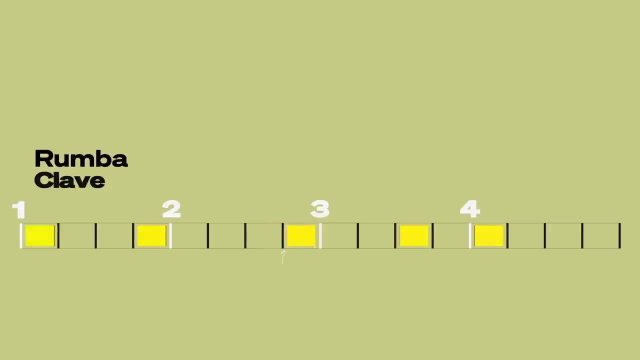 If you delay the third note by one sixteenth note, it's now known as Rumba Clave. Both of these are known as Three-Two Clave because three notes happen on the first half and two notes happen on the second half. By switching sides we now have Two-Three Rumba. 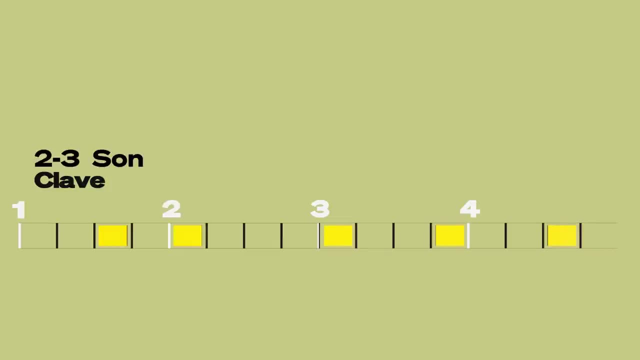 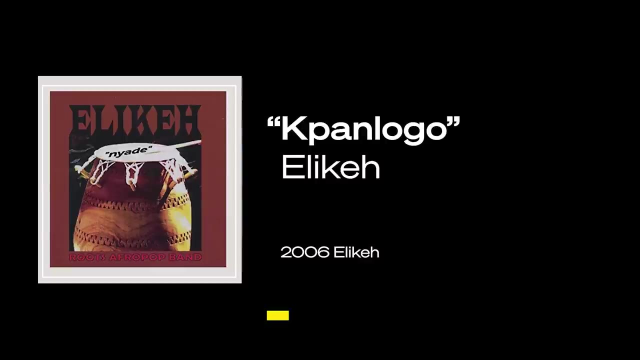 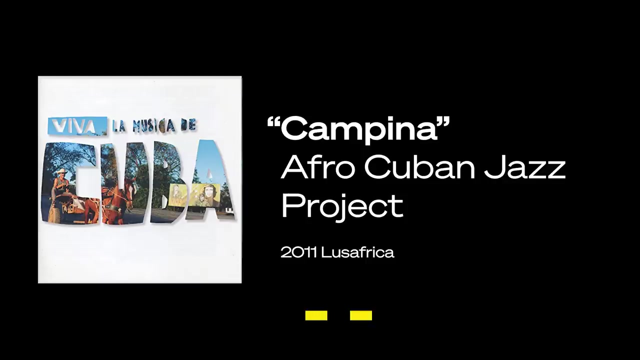 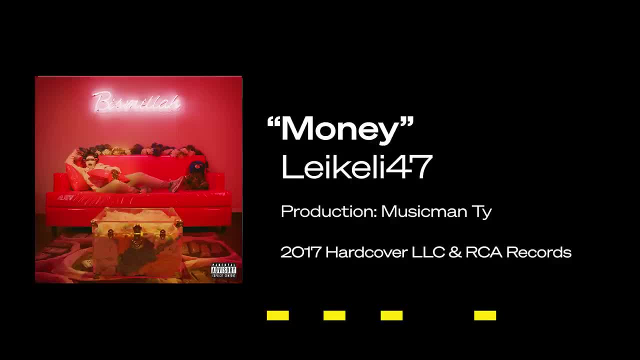 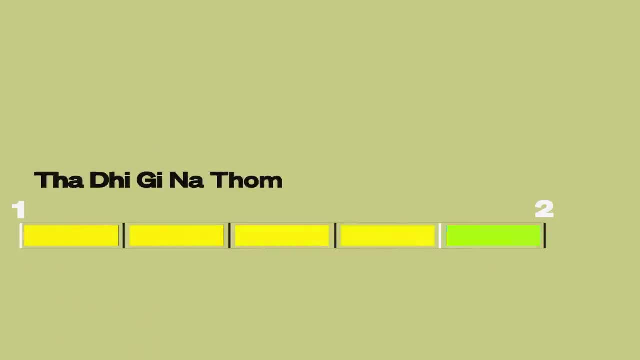 »Music playing ». »Music playing ». The last rhythm that changed my life is known as Tati Gin na Tom. This rhythm is part of the South Indian tradition known as Sol Kattu, which is a spoken rhythmic language in Carnatic music.